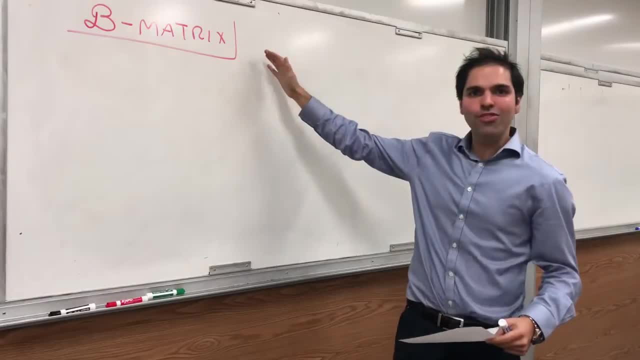 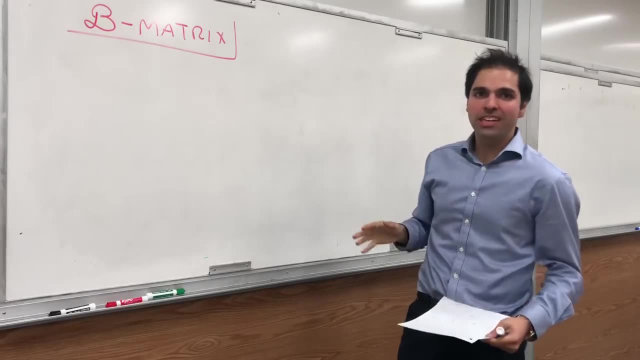 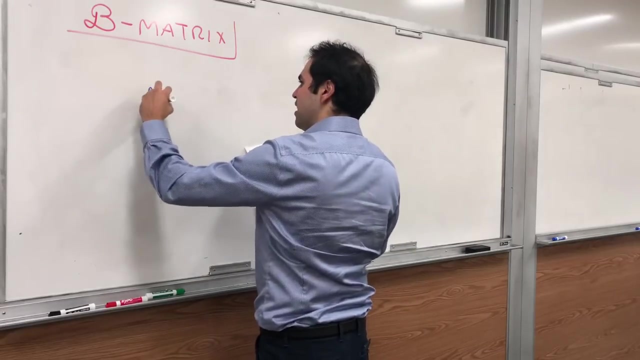 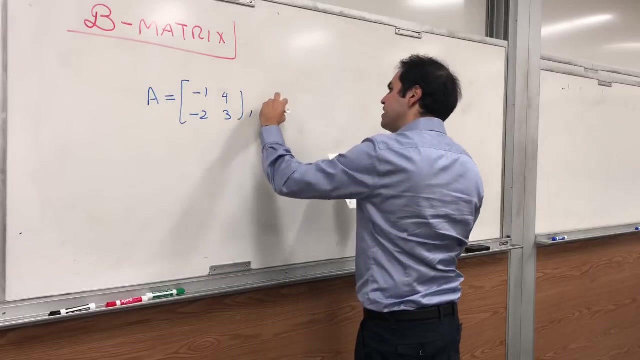 All right, thanks for watching. And today I want to find the matrix of a linear transformation with respect to a basis, B, Or, if you'd like, it's called the B matrix of A. Here's what I mean. So let A be the matrix minus 1,, minus 2,, 4,, 3.. And B be the basis. So beautiful B. 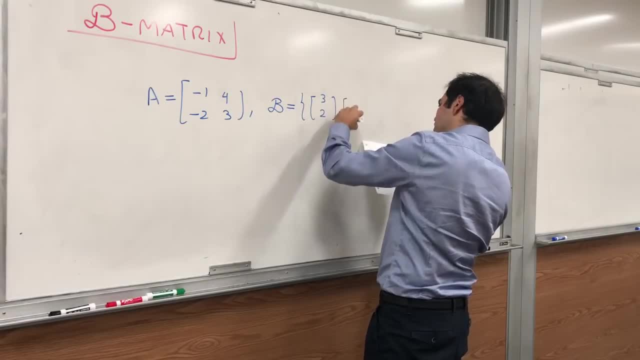 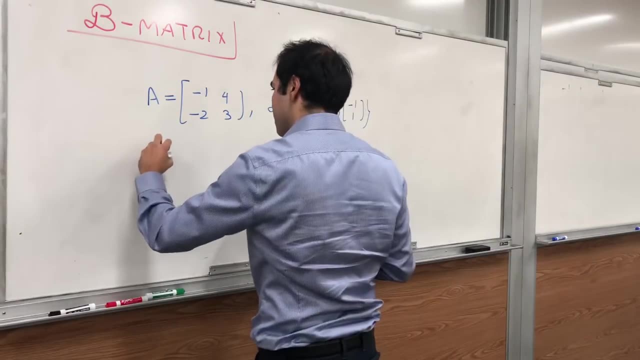 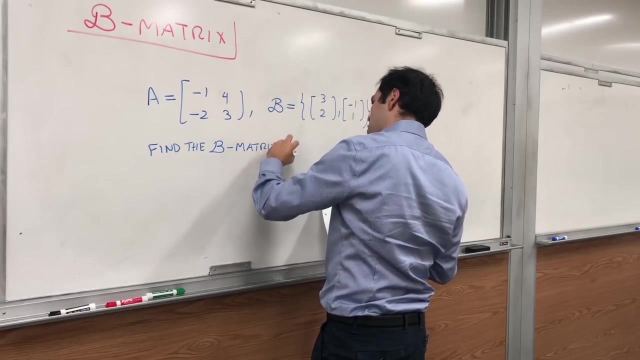 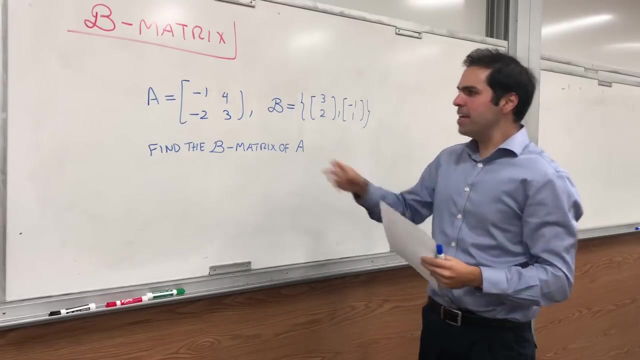 be the basis 3, 2, minus 1, 1.. And the question is: find the B matrix of A, B matrix of A. What does that mean? It really means find the matrix of the linear transformation T of X. 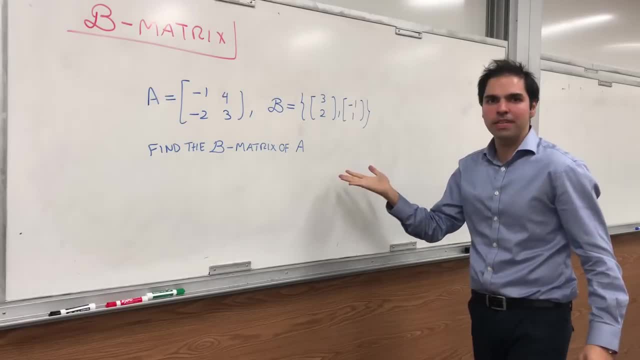 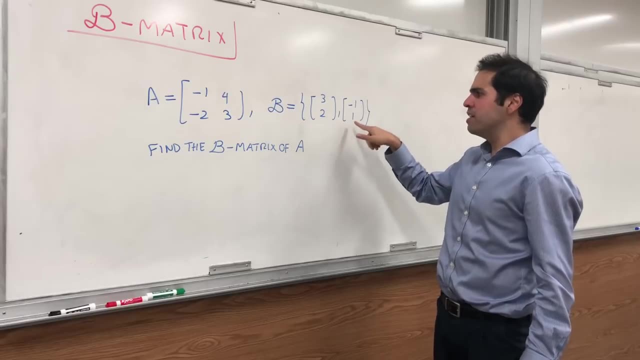 equals AX. What does that mean? It really means find the matrix of the linear transformation T of X with respect to the basis B. Now remember how to find matrices of linear transformations For every vector in the basis, you have to calculate T of that vector. So here let's. 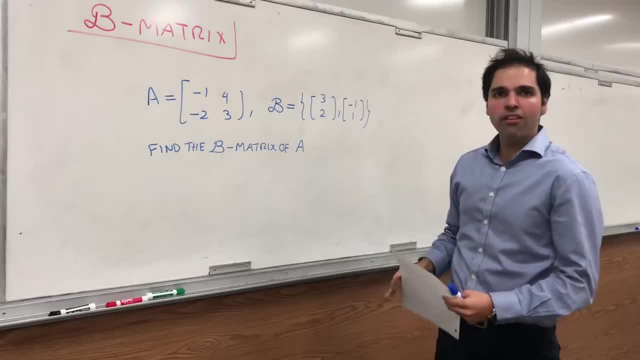 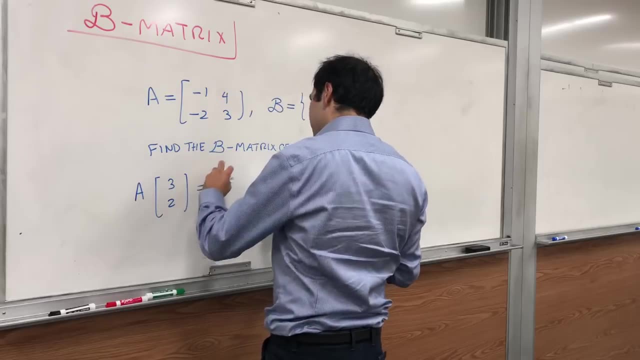 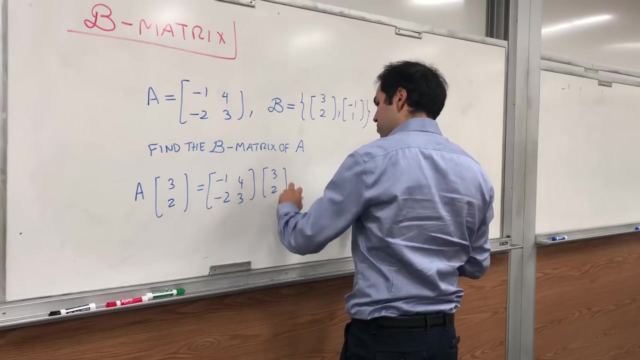 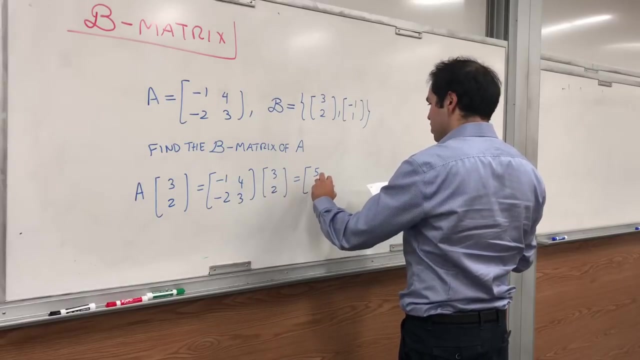 calculate A of 3, 2 and A of minus 1, 1.. So A of 3, 2.. Well, that's minus 1, minus 2, 4, 3.. 3, 2. And if you do that, you get minus 3 plus 8,, which is 5.. And minus 6 plus 6,, which is 0. 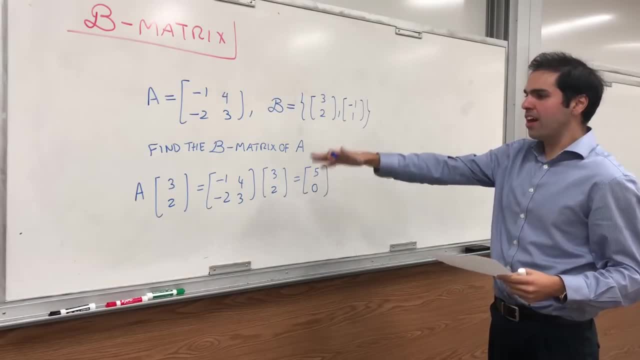 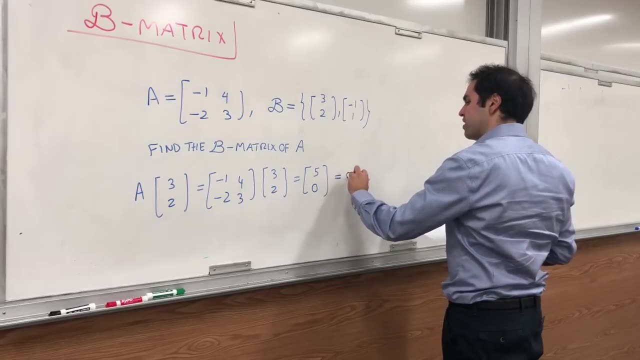 That's on the one hand. On the other hand, well, you calculated A of that vector. Now you just want to express it in terms of B, Think in terms of coordinates. So find the coordinates of this vector with respect to this basis. 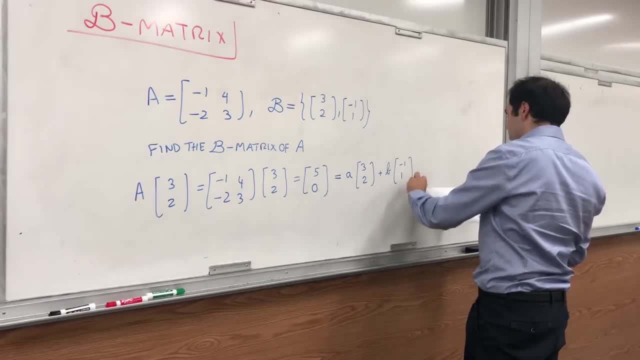 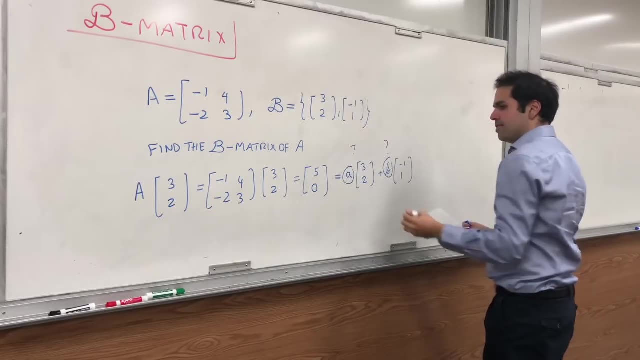 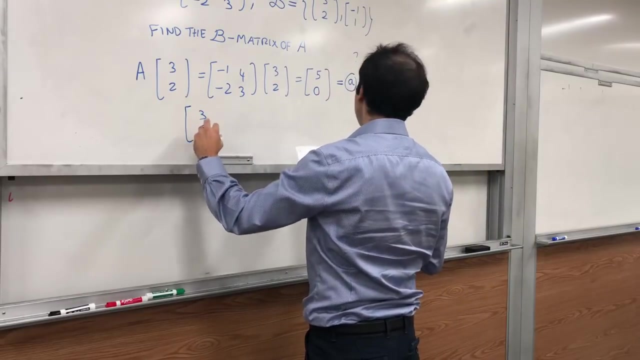 A times B, A times B, A times B, A times 3, 2 plus B times minus 1, 1.. And we want to find those coefficients, And so for this, you'll see, we just have to re-reduce a system. So do 3, 2, minus 1, 1, and then 5, 0.. Fortunately, 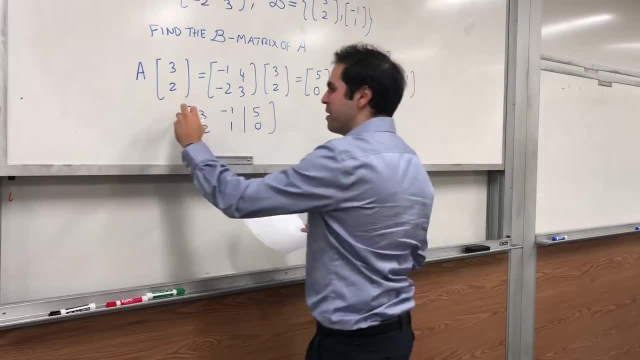 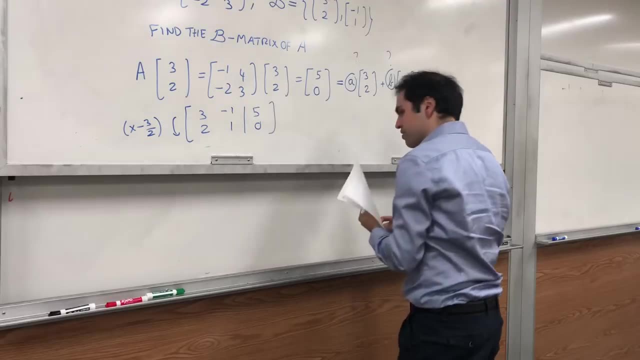 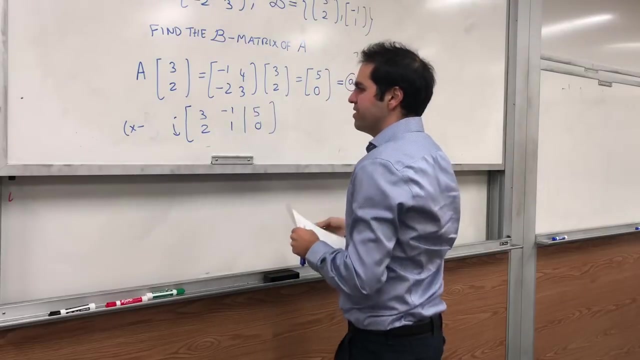 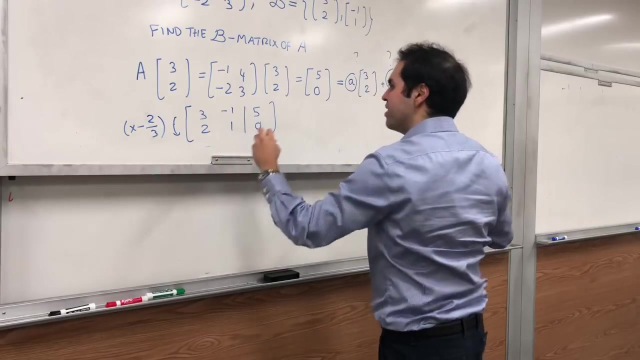 there isn't a very clever way of doing this, So just do it by brute force. So let's multiply the first row by? I think. no, Let's multiply the first row by minus 2 thirds And add it to the second row, Because minus 2 thirds is the thing that transforms 3 into minus 2.. And that's what. 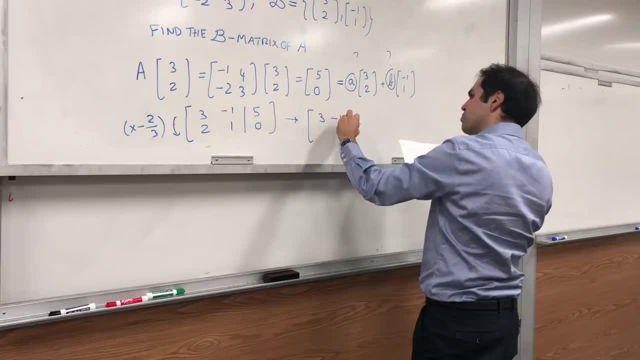 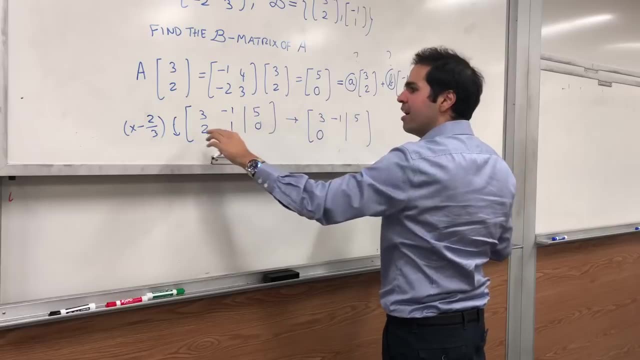 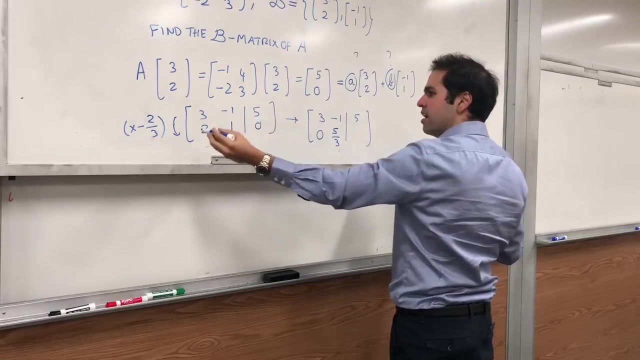 we want. Then we get again 3 minus 1, 5. And then 3 times minus 2 thirds, That's minus 2 plus 2.. It's 0.. Minus 1, times minus 2 thirds: It's 2 thirds Plus 1. It's 5 thirds. And then 5 minus 2 thirds, It's minus 10. 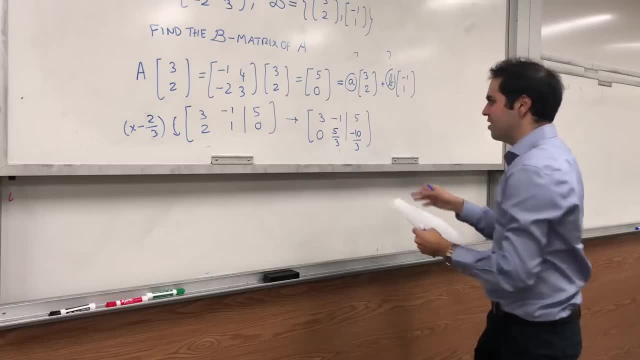 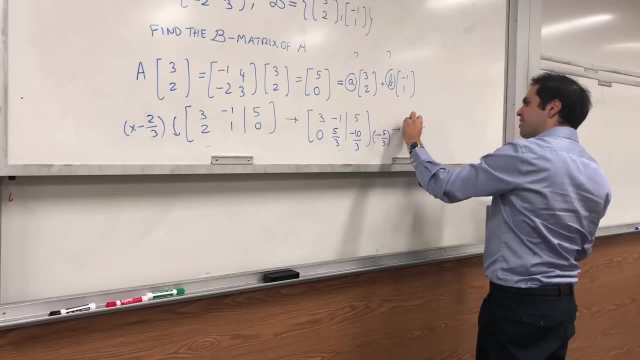 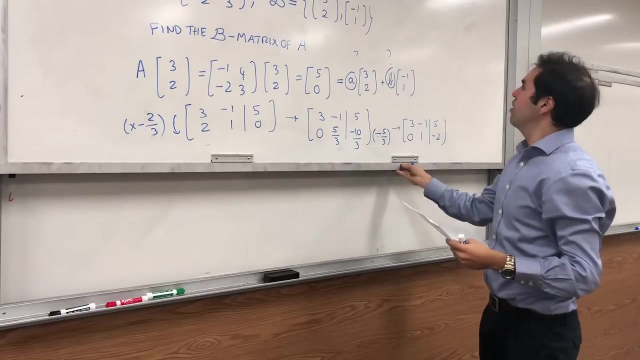 thirds Plus 0.. It's minus 10 thirds. But notice, this simplifies quite nicely. You can divide by 5 thirds And you get 3 minus 1,, 0, 1.. 5 minus 2.. And then let's just continue re-reducing, So we get. 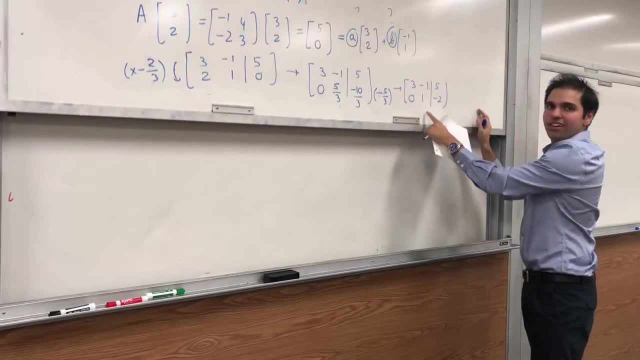 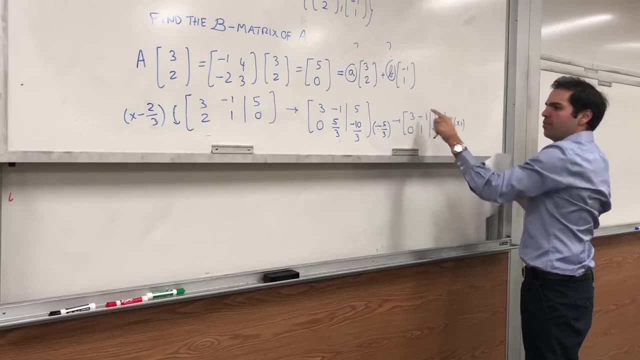 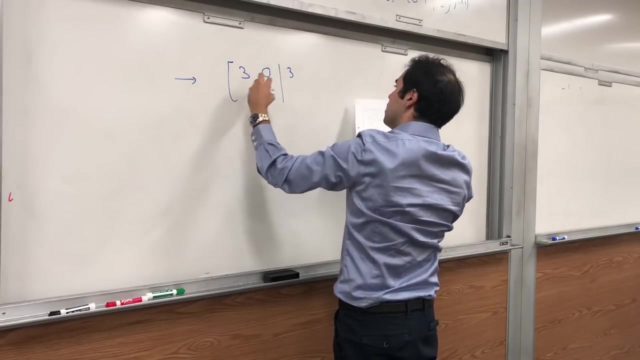 1, 0, 1, 0, 1, minus 2.. So I mean it is in row echelon form, But let's make it into reduced row echelon form. So let's add the second row to the first row And we get 3, 0, 3, 0, 1, minus 2.. And 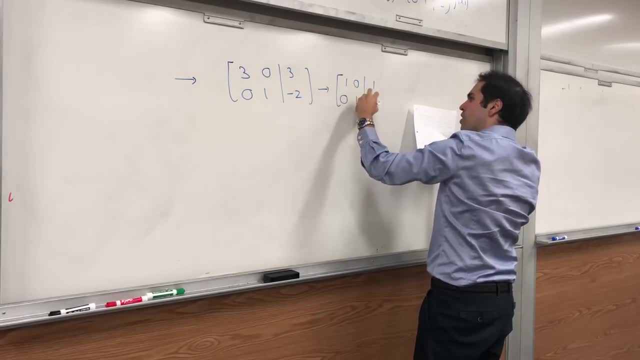 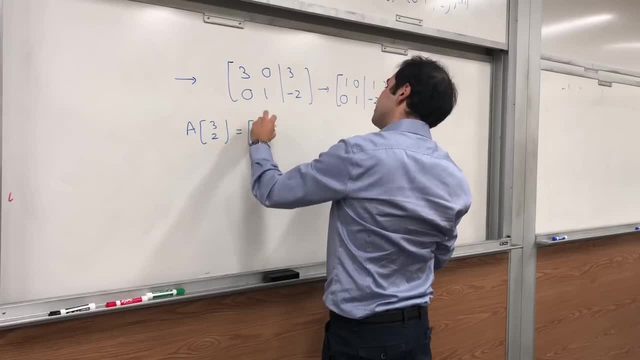 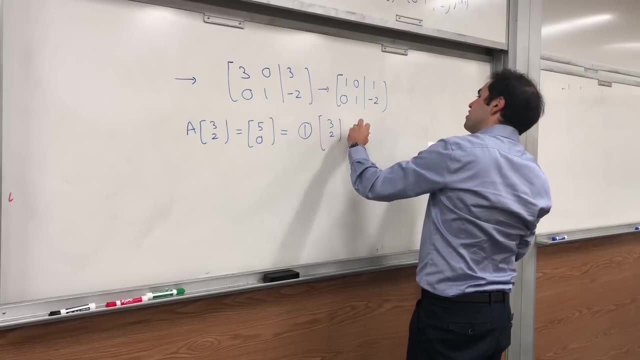 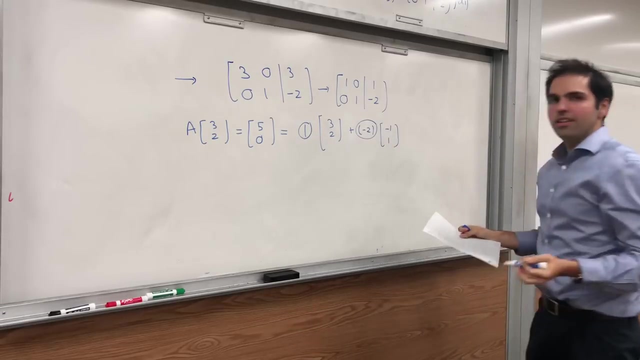 B of 3, 2,, which is 5, 0,, equals to 1 times 3, 2, plus minus 2 times 5, 0, times minus 1, 1.. And just like for matrices of linear transformations, all you do, you take those. 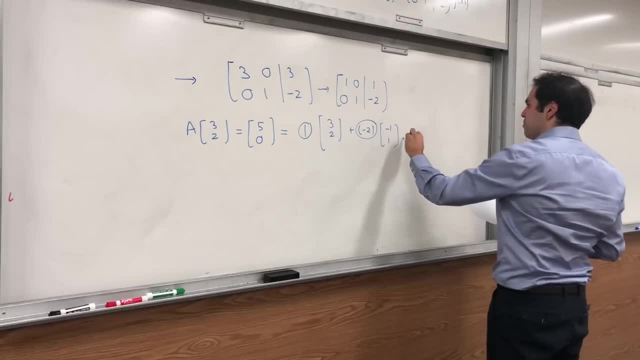 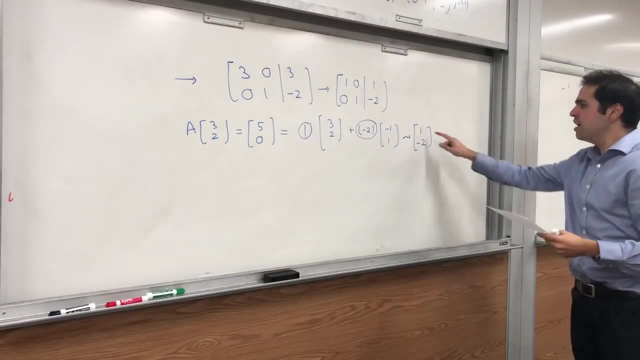 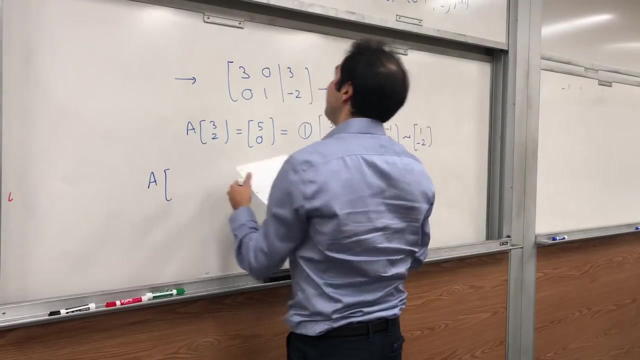 two coefficients together and put them in a column, in a column vector. So in other words, we know that that the first column of the B matrix of A is 1 minus 2.. And then for the second vector, for the second column, 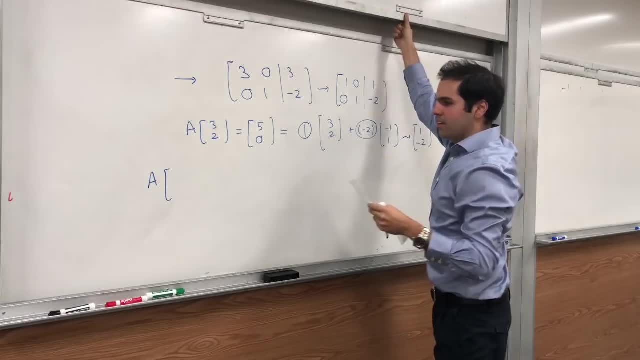 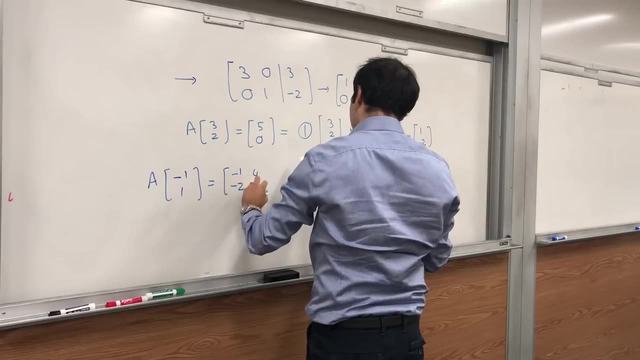 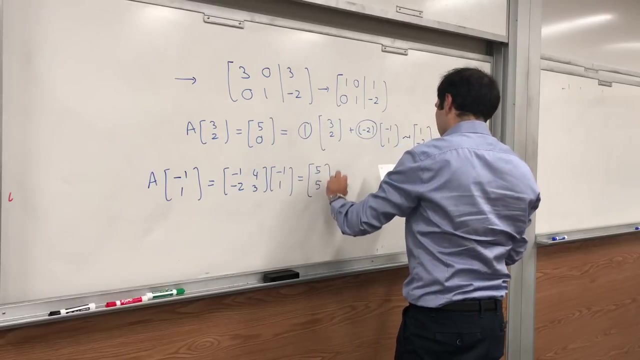 you do A of minus 1, 1, calculate that, So it's minus 1,, minus 2,, 4, 3, and minus 1, 1.. And if you do that you get 5, 5.. 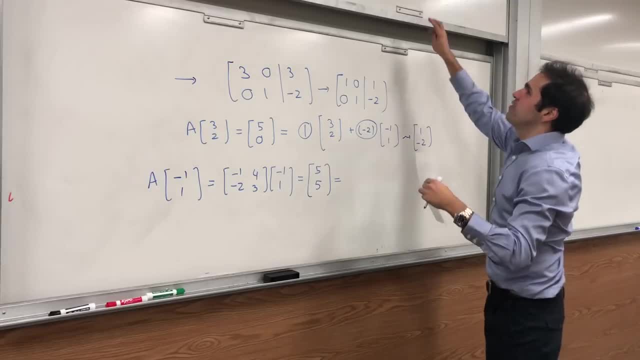 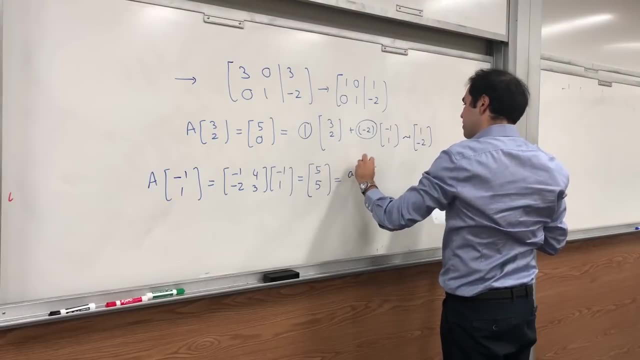 And again, just as before, you want to write this in terms of your basis vectors 3, 2, and minus 1, 1.. So it's A times 3, 2 plus B times minus 1, 1.. 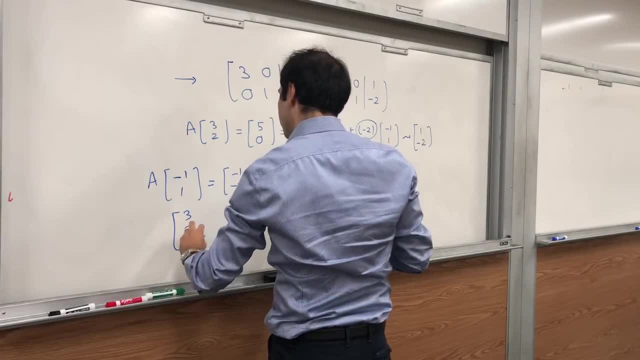 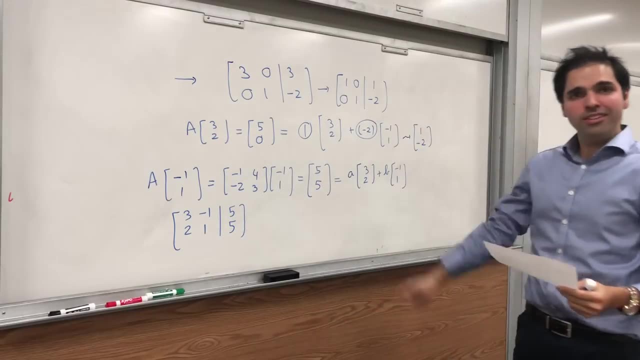 And, just as before, you just need to row reduce the matrix 3, 2, minus 1, 1, 5, 5.. And I'm not going to do this again, because it turns out it's the exact same process. 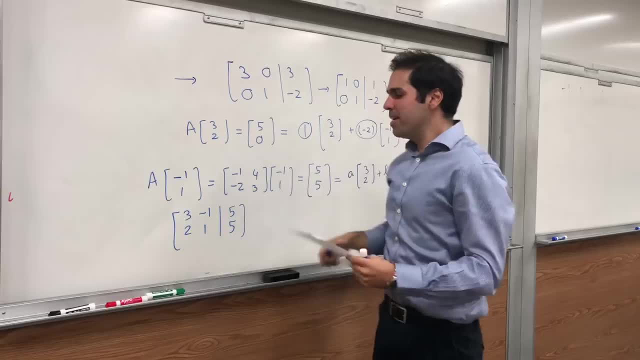 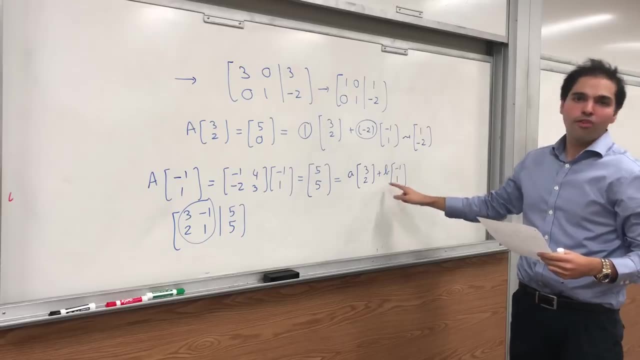 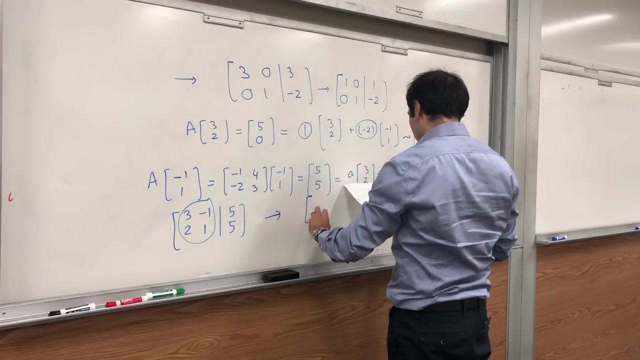 You use the exact same row reductions because, notice, this matrix is actually the same as before And it's just a matrix formed by putting the columns of B together. So if you do that, after a while you should get, I think, 1, 0,, 0, 1, and 2, 1,. 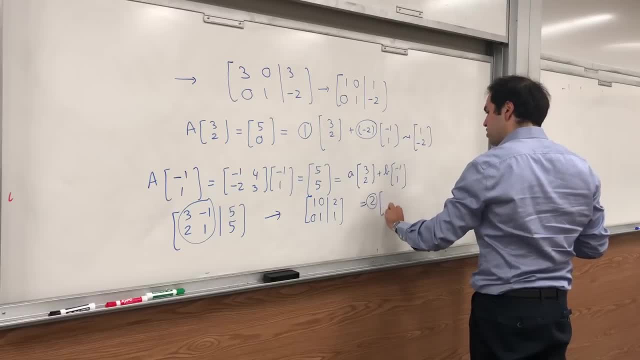 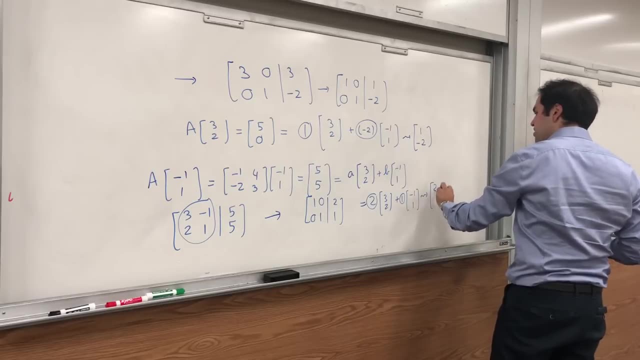 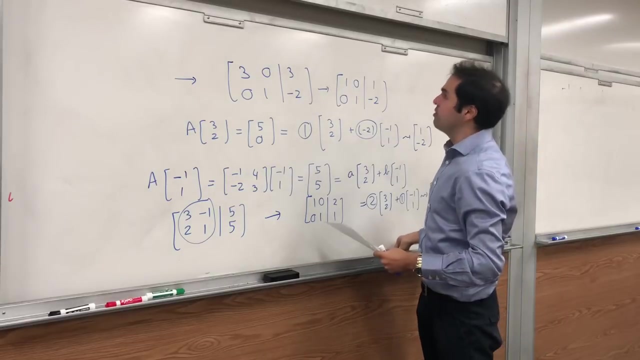 which tells you the answer is 2 times 3, 2 plus 1 times minus 1, 1.. And therefore the second column of your matrix is 2, 1,, which tells you, in the end, what is the B matrix of A. 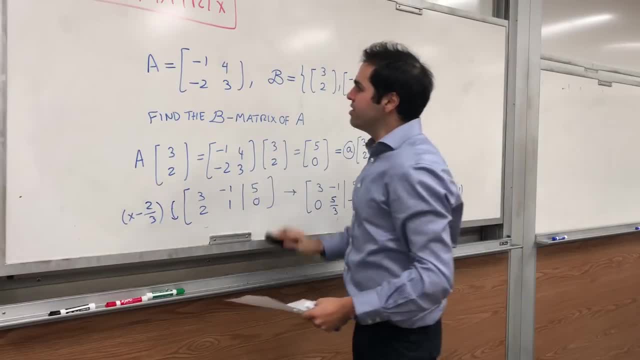 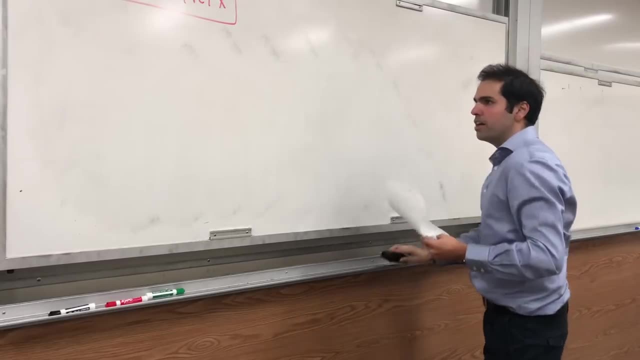 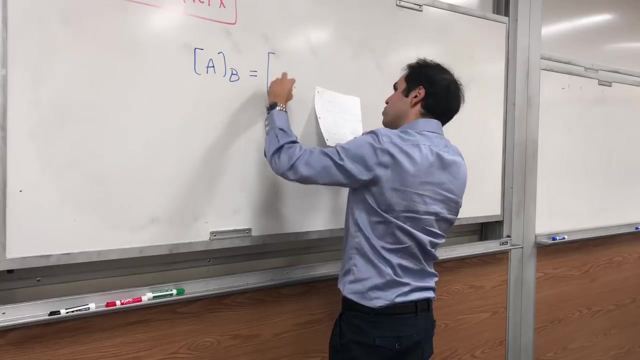 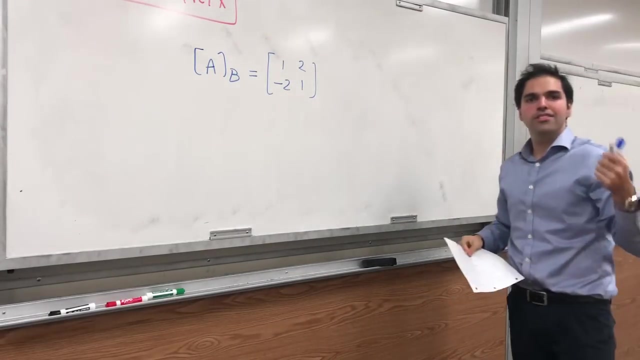 It's just the result you get by putting those two vectors together. So let's just write it as follows: So AB equals to 1 minus 2, 2, 1.. And you see, it's a very similar process to finding matrices of linear transformations. 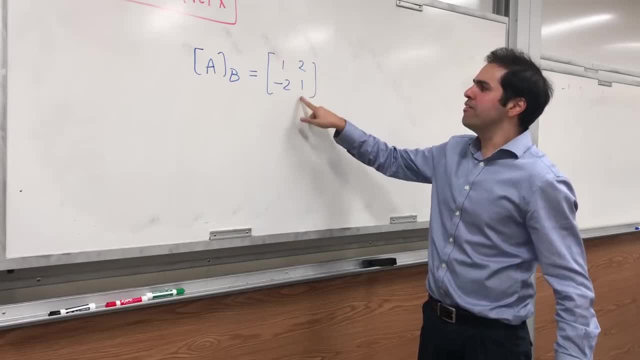 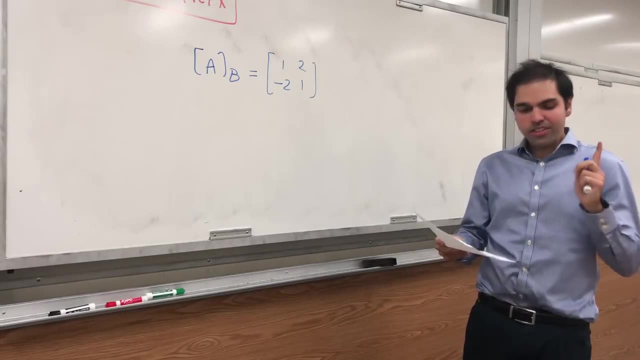 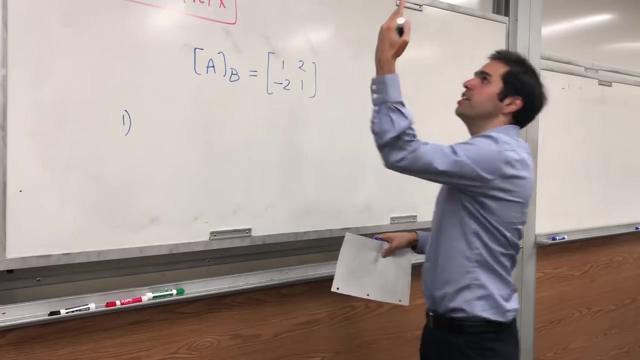 For linear transformations. for every vector, you evaluate t of that vector and you express it in terms of the vectors you've got. So Just a couple of notes, though, First of all here. we did it in a slow way. 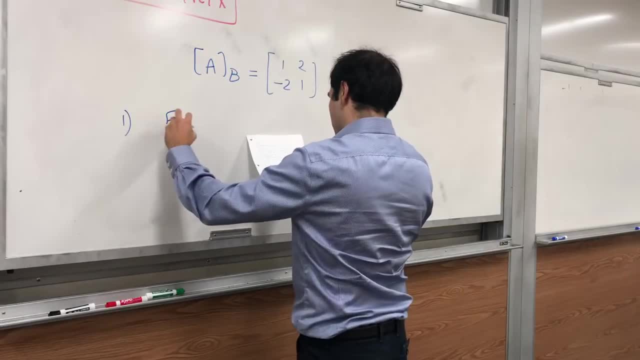 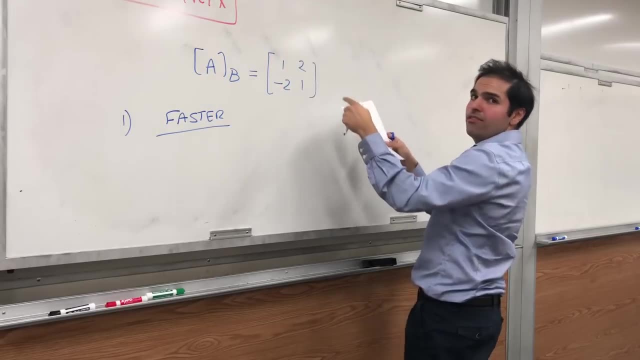 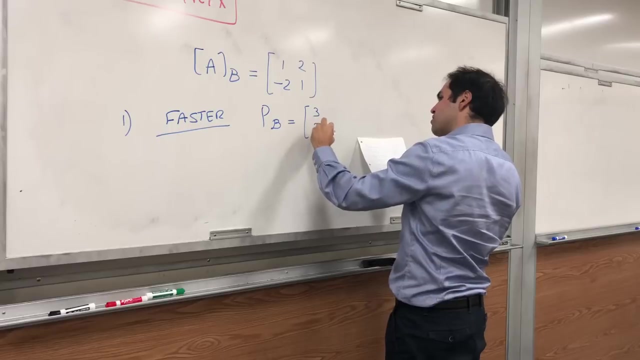 There's actually a much faster way to do this. So remember, if you put the vectors in B together, you get what's called the change of coordinates matrix PB, which is 3, 2, minus 1, 1.. 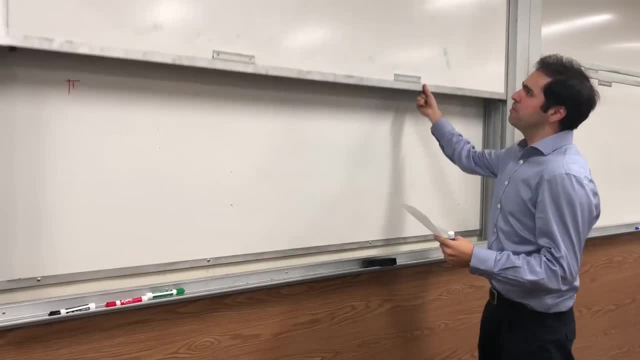 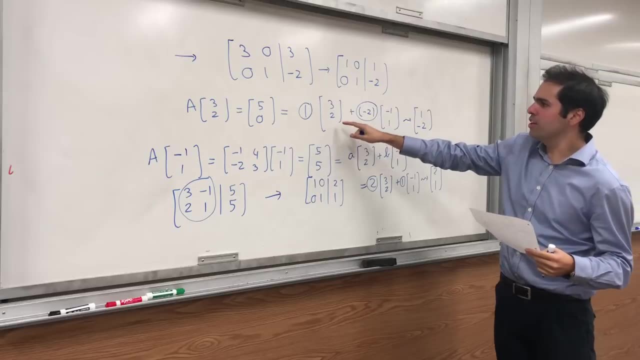 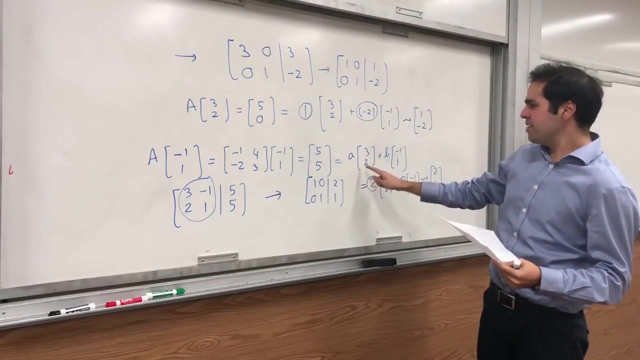 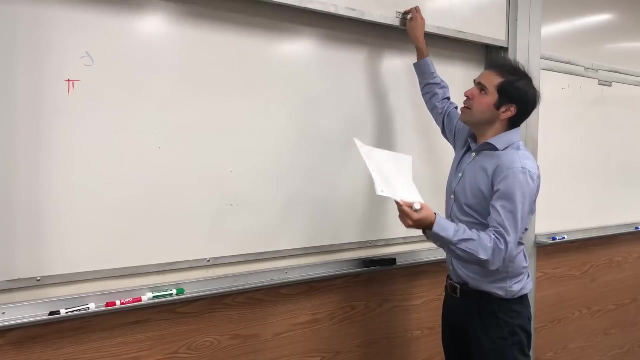 And notice what we really did in this problem. For example, here we tried to solve PB of what and what gives you 5, 0.. Similarly, here, PB of what and what gives you 5, 5.. So really all we needed to find under following, namely: 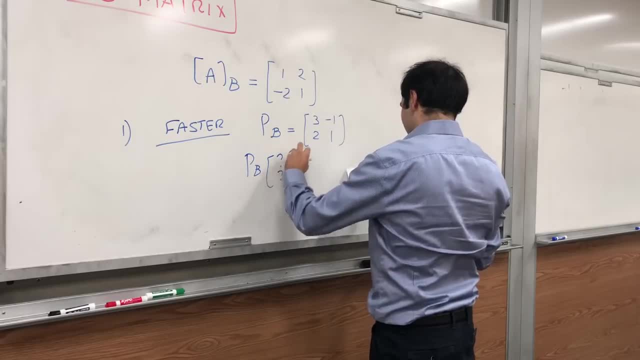 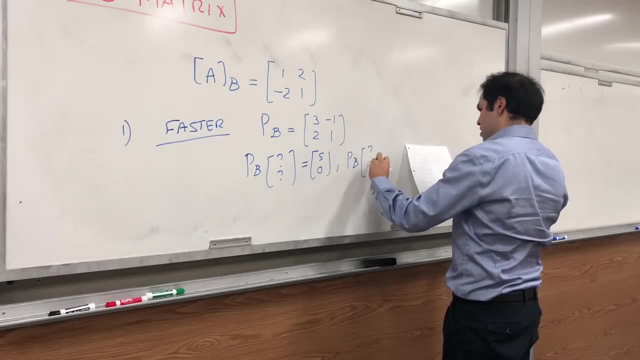 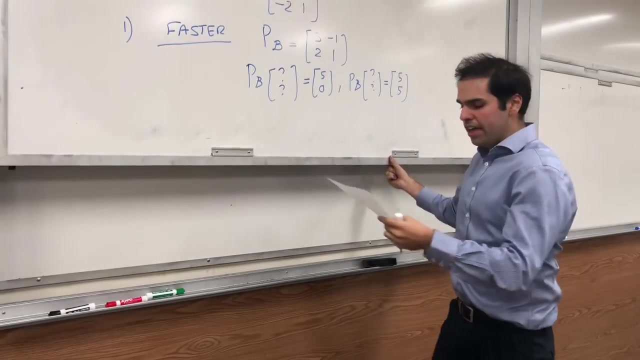 PB of what and what of what-what. what-what gives you 5, 0.. And Pb of what-what gives you 5,, 5.. And so, really, all you needed to do is to take Pb in the first column. 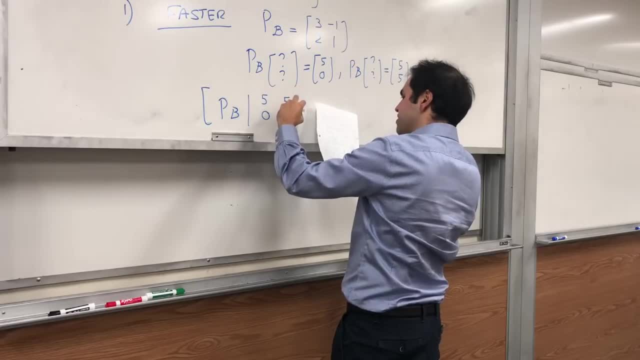 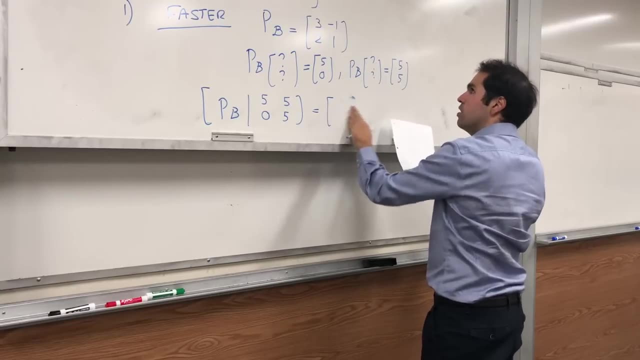 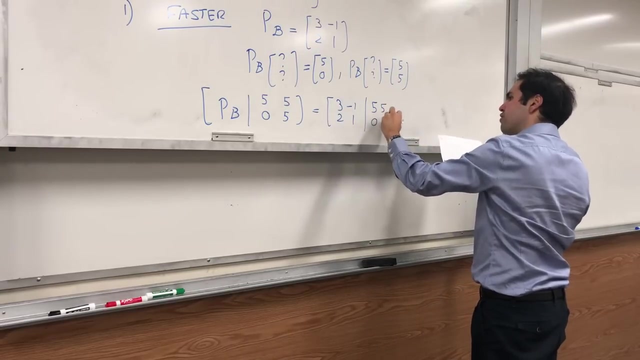 and a of the first vector, a of the second vector, which is, just you know, 1 minus 2, 2, sorry, Yeah, no- which is 3, 2 minus 1, 1, and 5, 5, 0, 5.. 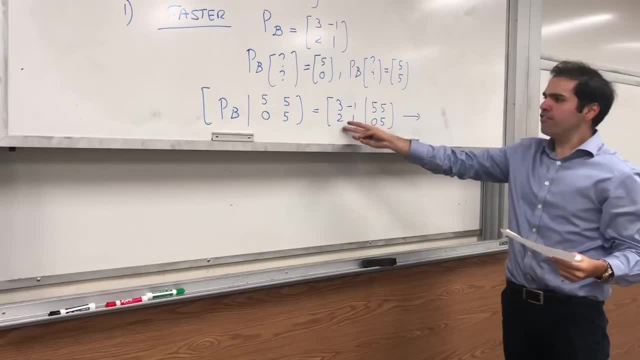 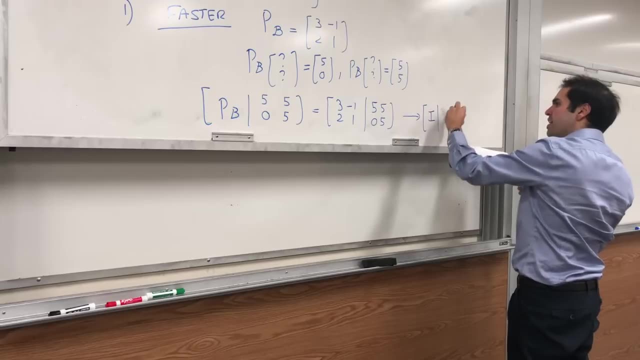 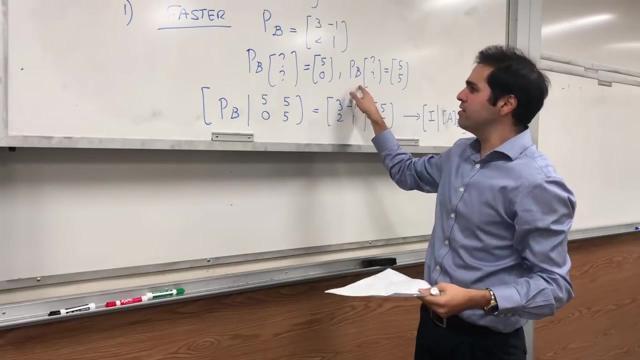 And just row reduce it so that the left-hand side is the reduced row echelon form, which here means the identity matrix I, N, A, B, And that just reflects that in both cases We use the exact same row. you know row reductions. 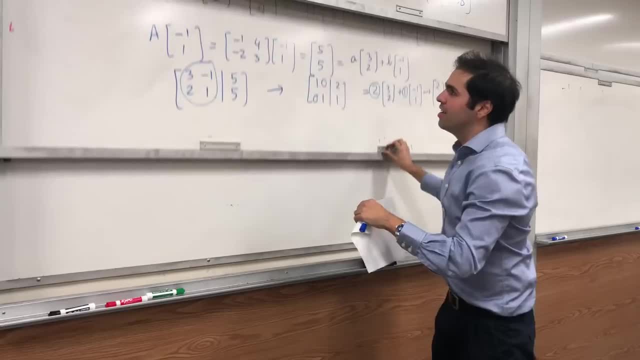 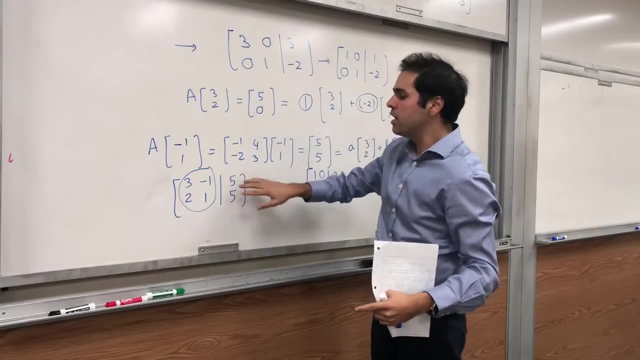 Because notice in fact, in those two things- again the stuff I erase in here- we started out with the same matrix, which is Pb. It's just the right-hand side that changed a bit And we tried to make the left-hand side. 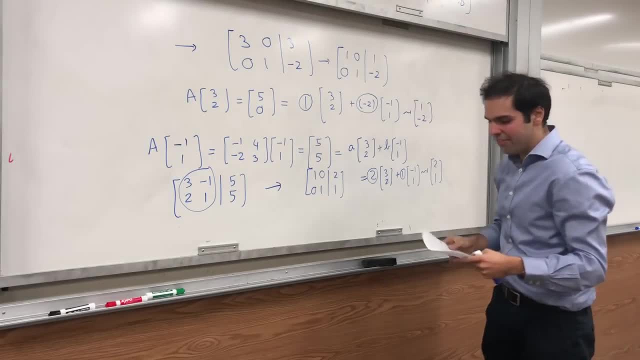 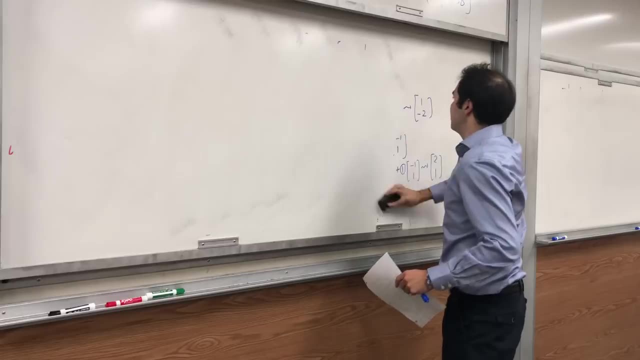 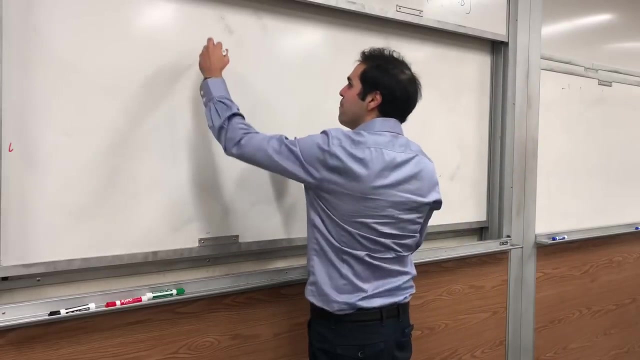 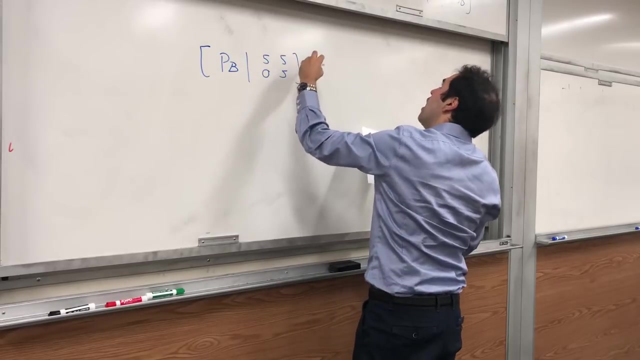 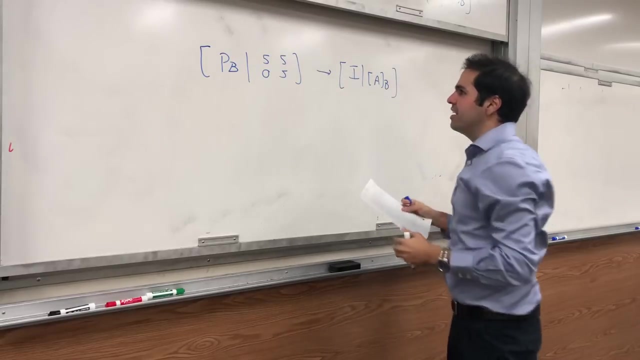 be the identity matrix, which is precisely what we have here, And also I want to emphasize this because I think this is important. So we had Pb and then 5, 0,, 5, 5, and it gave us I N, A, B. 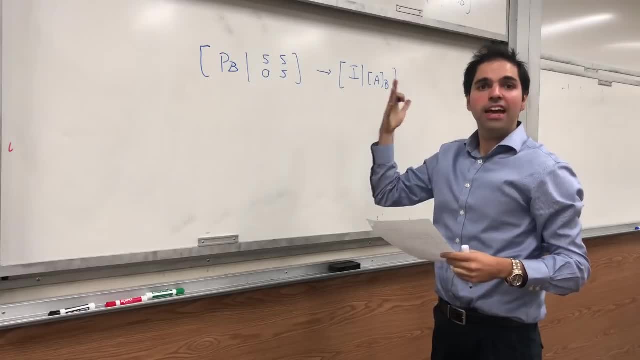 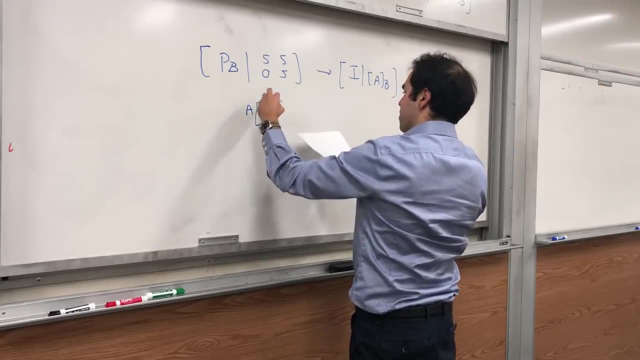 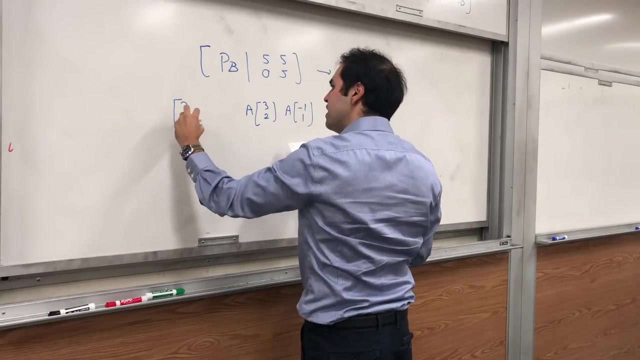 Now, how did we find this matrix? We applied A to every basis, Every basis vector, So this was really A of- let's see- 3, 2.. And this was A of minus 1, 1.. And remember, Pb was just a matrix. 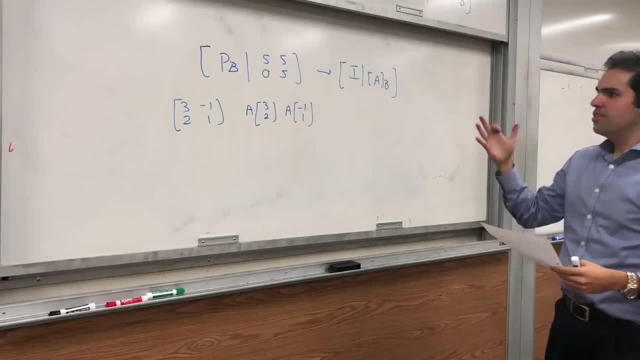 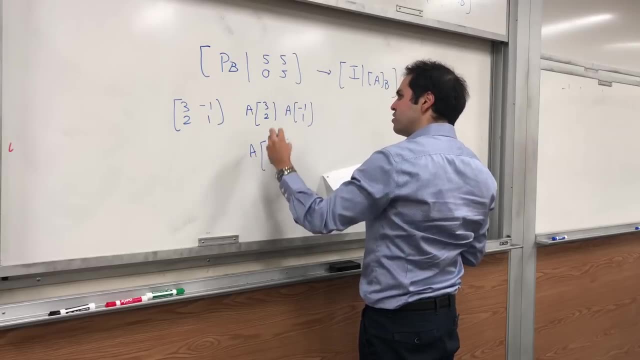 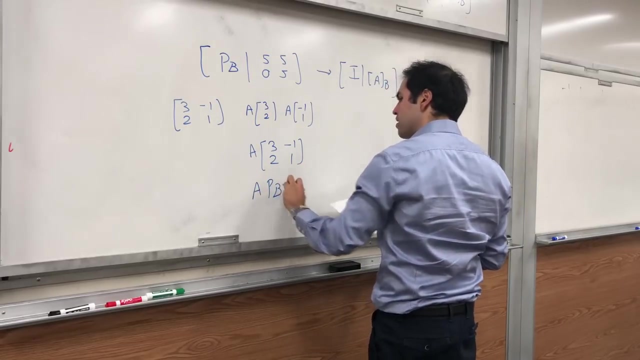 by putting all the vectors in B together. So notice: this thing is just the same as A applied to the matrix 3, 2 minus 1, 1, which is really A Pb, Because this is precisely the matrix P. 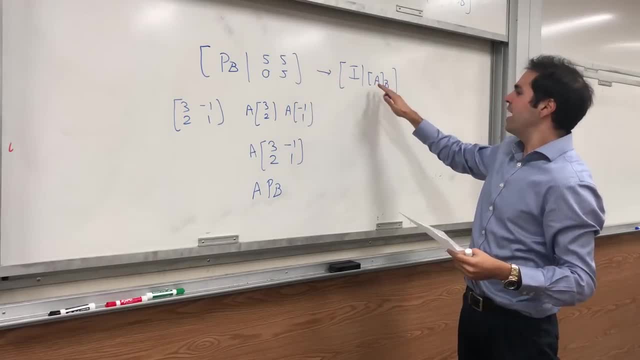 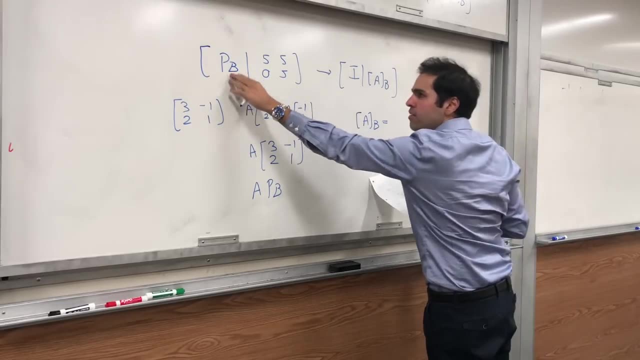 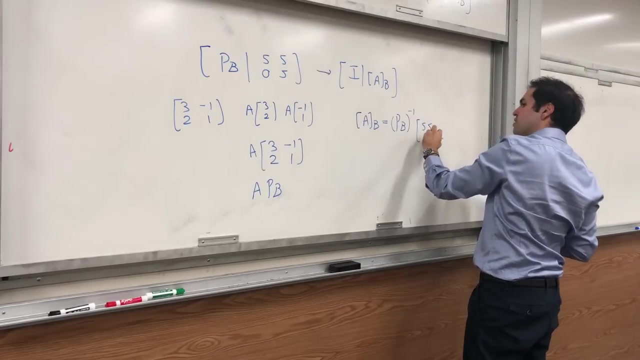 And what did we do? Well, really, we just tried to invert it. So, really, A, B is the result of inverting Pb applied to this matrix 5, 5, 0, 5.. Which was what was this matrix? 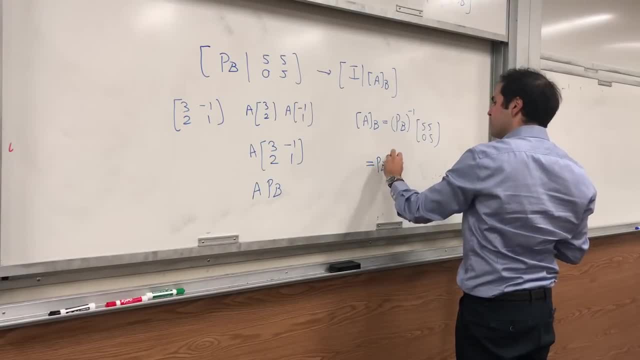 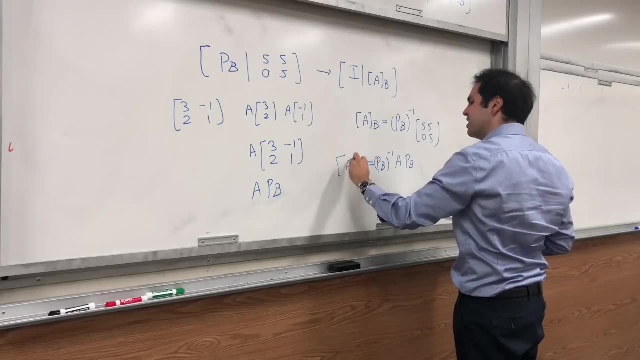 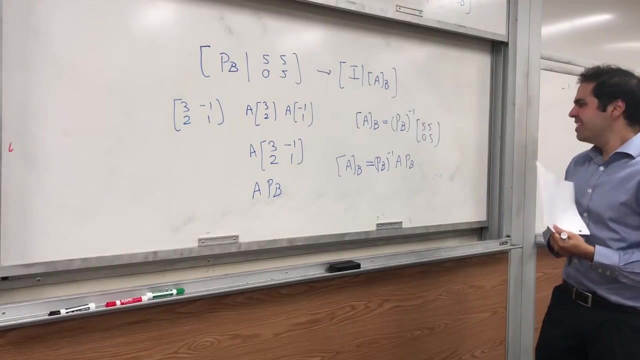 A of this, So A of A of Pb. So this is really cool To find the matrix, the B matrix of A. we did something similar to diagonalization, We. this is called conjugation by Pb And this is why, you know, we have this identity, you know. 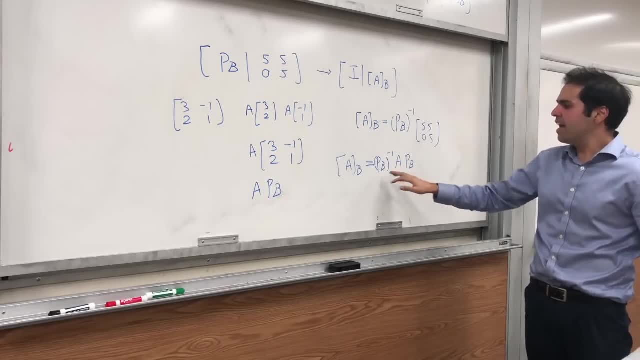 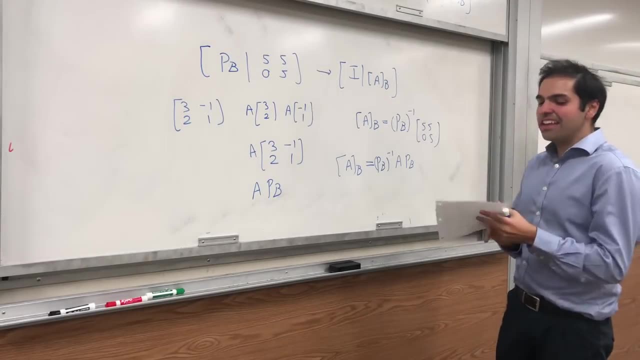 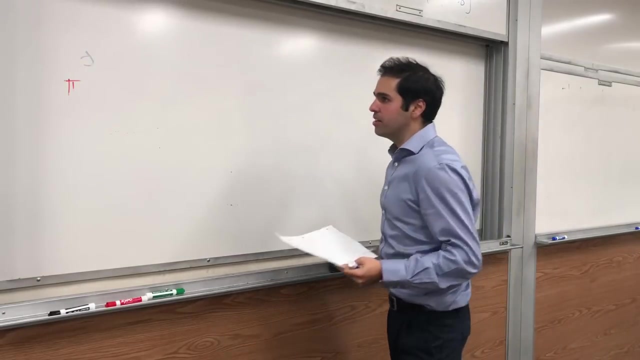 What's called the B matrix of A is just Pb A, Pb inverse. This is one cool thing, where sort of diagonalization comes in, And the real reason why this is important is as follows. In fact, let me try to do it on this last one. 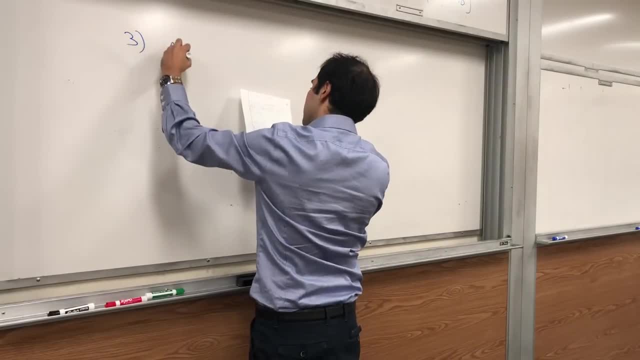 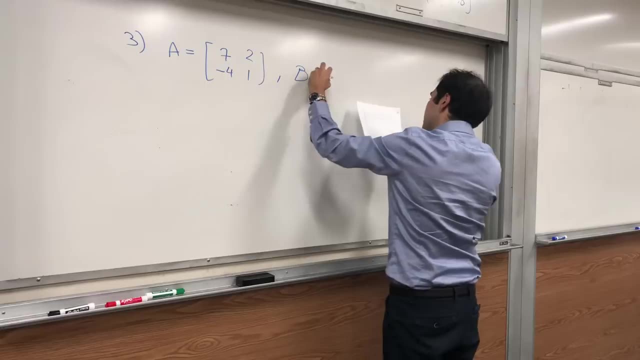 Suppose A is 7 minus 4 and 2, 1.. And B is 1, minus 1 and 1, minus 2.. What's this? So let's do it again. So, let's do it again. Let's do it again. 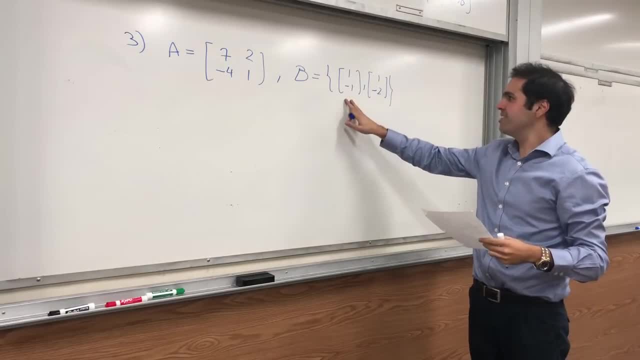 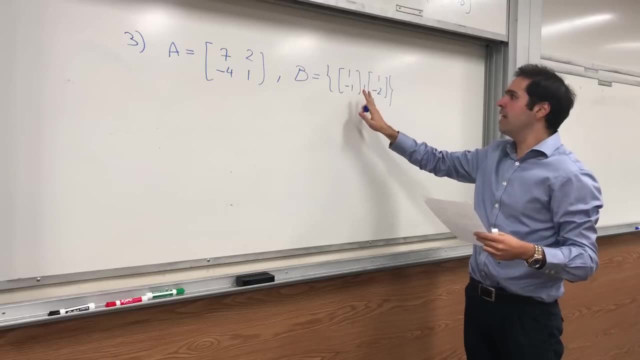 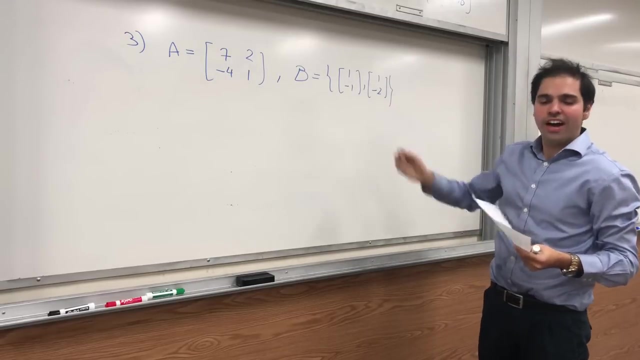 And I already want to tell you from the outset, those ones will be our eigenvectors of A. So the question is, what happens to the matrix of A if B- is you know the sorry- if B is you know- consists of eigenvectors. 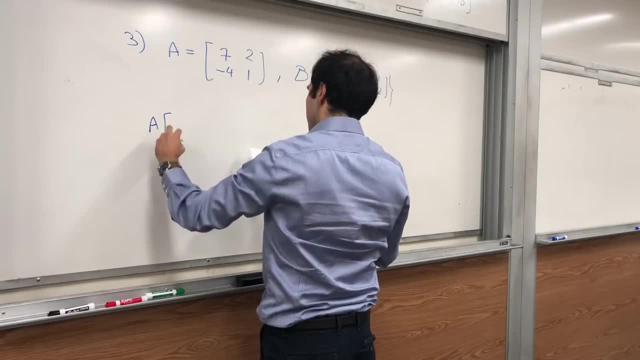 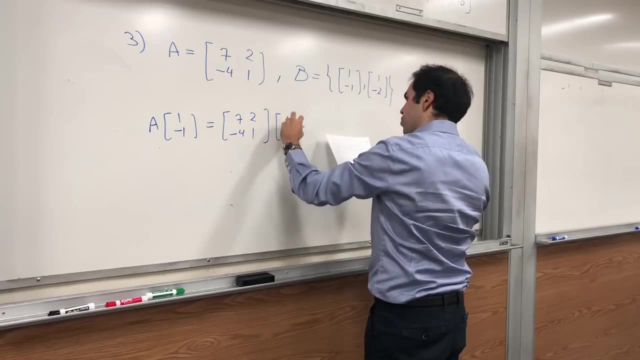 Well, let's do that. Let's calculate A of 1 minus 1.. Well, that's 7, 2, minus 4, 1, and 1 minus 1.. If you do that turns out it's 5 minus 5.. 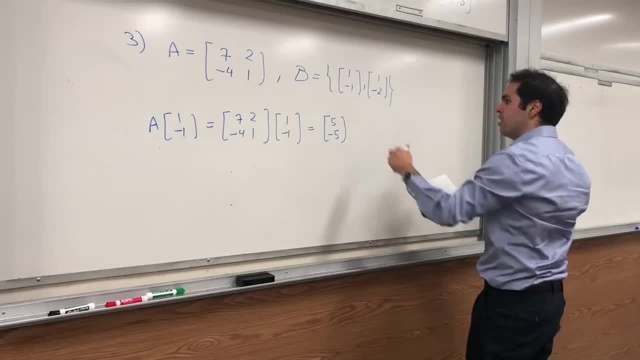 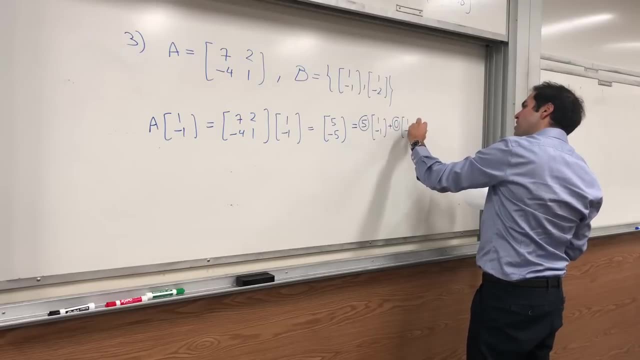 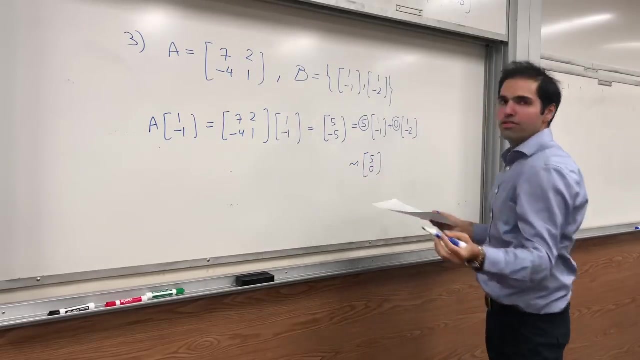 And now, how can you write it in terms of those vectors? Well, it is indeed 5 times 1 minus 1 plus 0 times 1 minus 2.. And indeed the column here becomes 5, 0.. The first column. 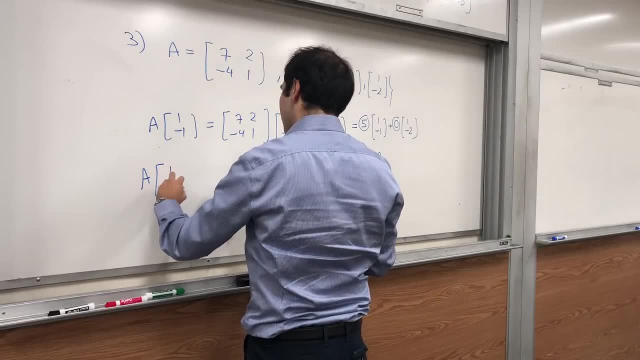 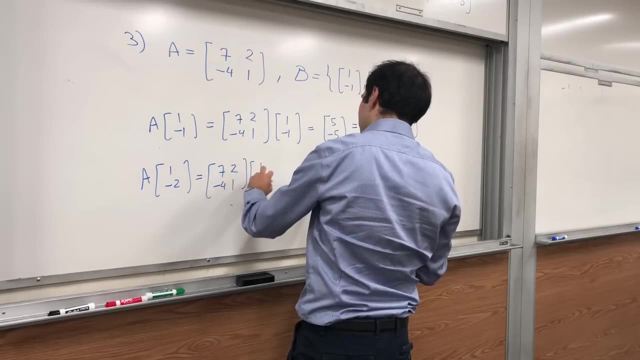 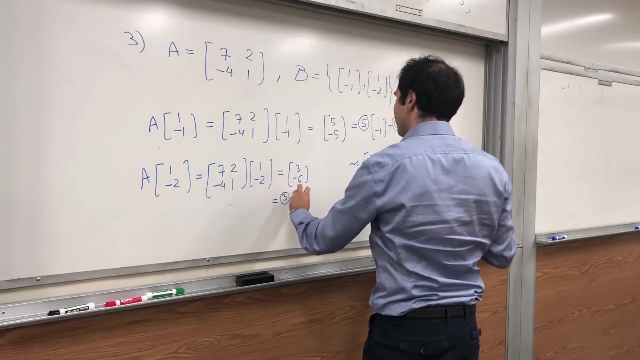 The first column of the B matrix, Now A of 1 minus 2, that is 7, 2, minus 4, 1, of 1 minus 2.. And that's 3 minus 6.. And again, write it in terms of your basis vectors. 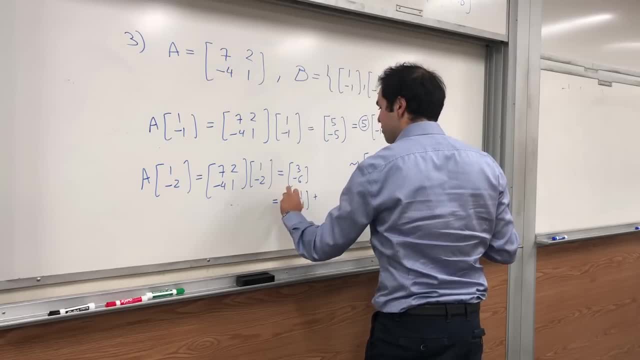 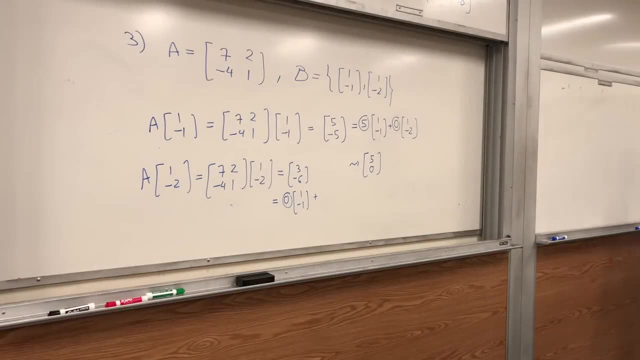 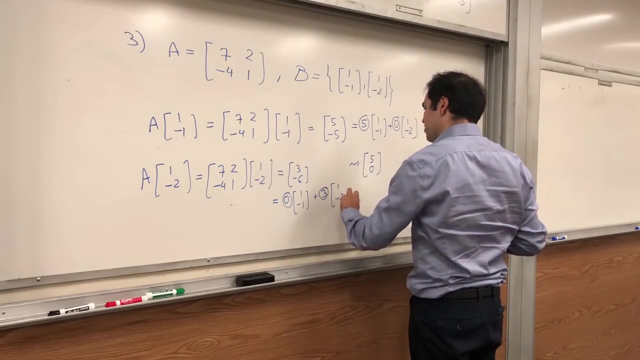 3 times 1 minus 1, sorry, 0 times 1 minus 1.. Woo, One second Not expected. Ah, I didn't know. Okay, 0 times 1 minus 1 plus 3 times 1 minus 2.. 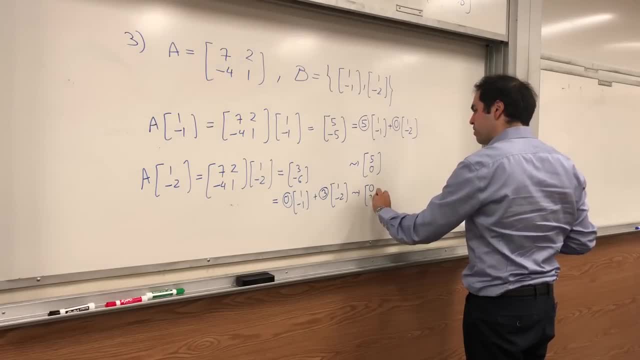 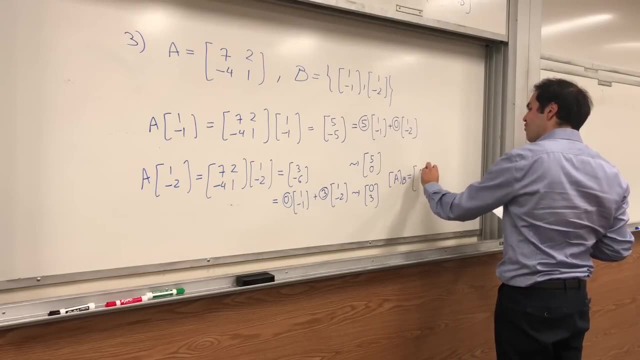 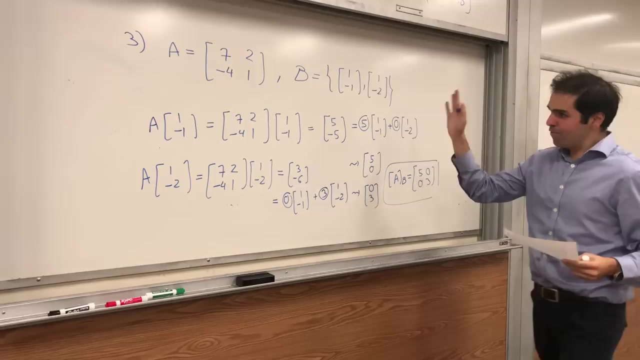 And therefore the second column becomes 0, 3.. Which means that the B matrix of A is 5, 0, 0, 3.. So you see, what made this work is that you know we had eigenvectors.